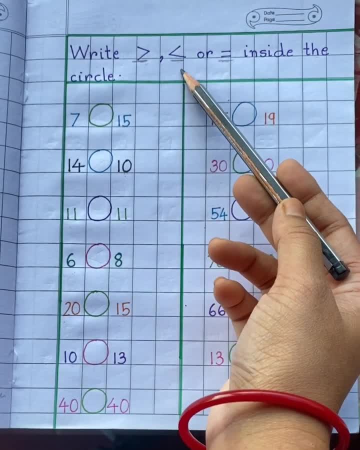 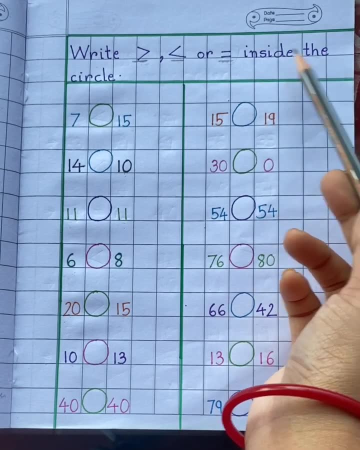 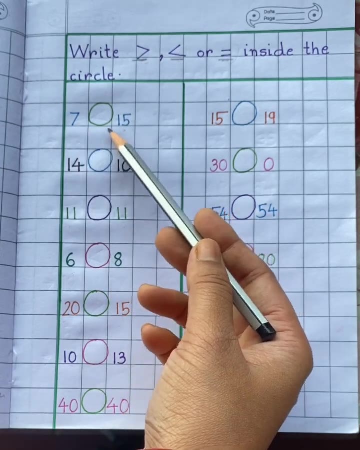 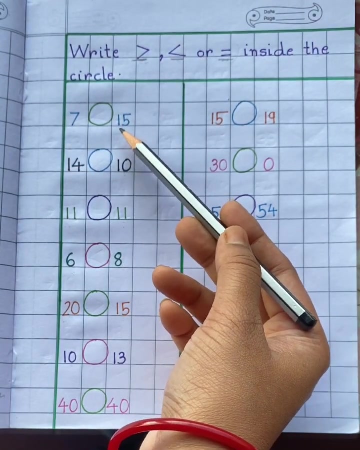 Less than this is the sign for less than or equal to. This is the sign for equal to inside the circle 7, 15.. While comparing these two numbers, which number is greater? 15 is greater, So we will put less than sign. 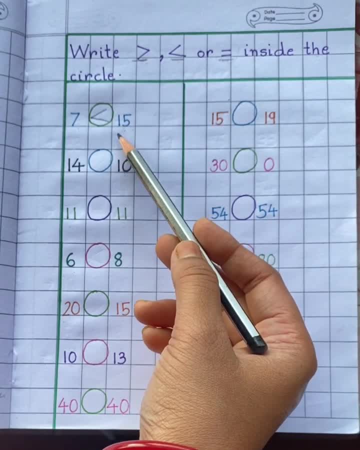 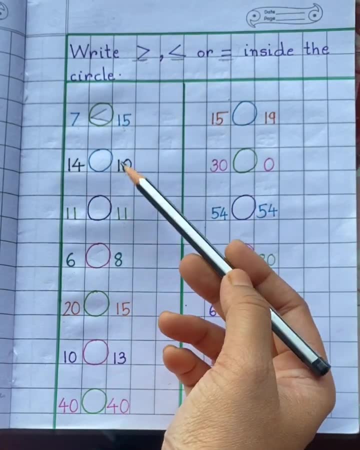 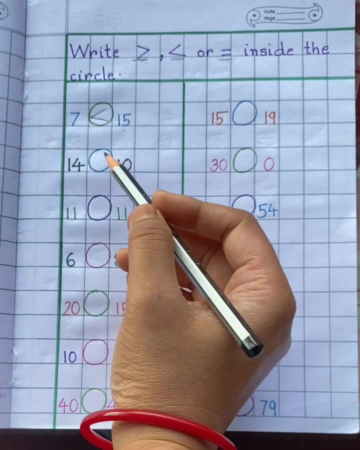 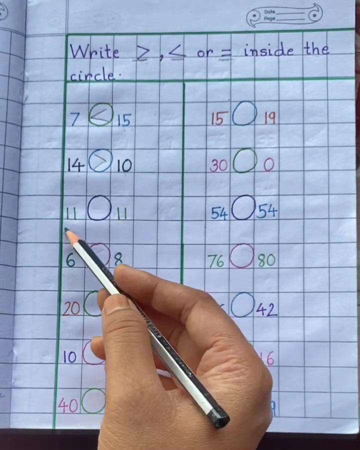 11 is less than 15.. 14, 10.. While comparing these two numbers, which number is greater? 14.. 14 is greater than 10.. So we will put greater than sign 11, 11.. Both the numbers are same. So what sign we are going to put now? 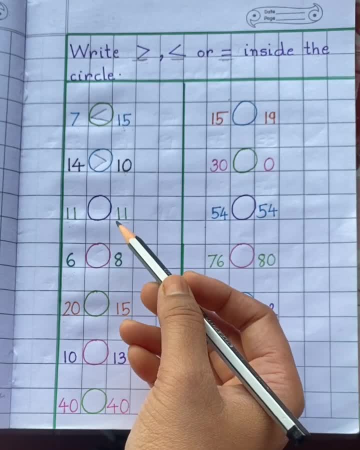 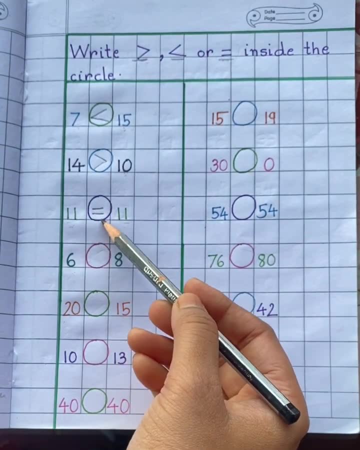 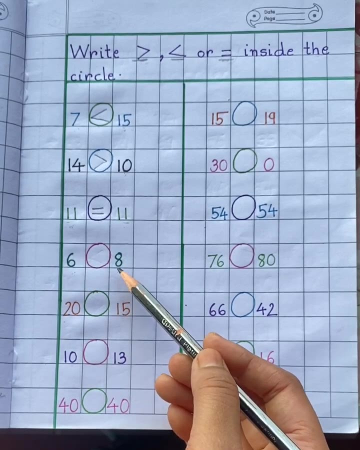 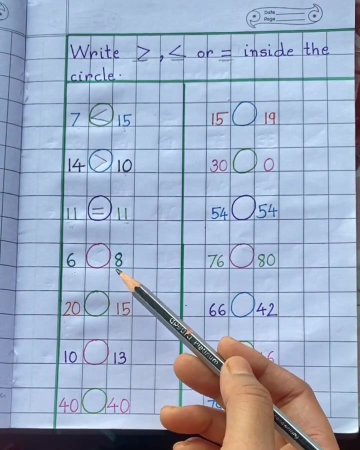 If both the numbers are same, we are going to put equal to sign. So we will say 11 is equal to 11.. Next numbers are 6, 8.. While comparing these two numbers, which number is greater? 8.? 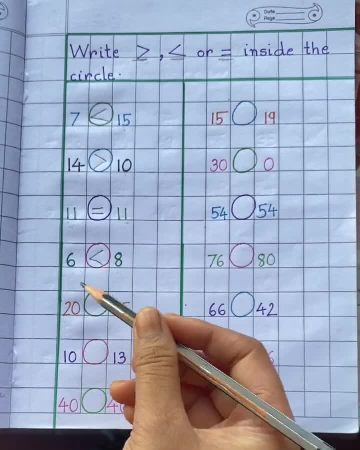 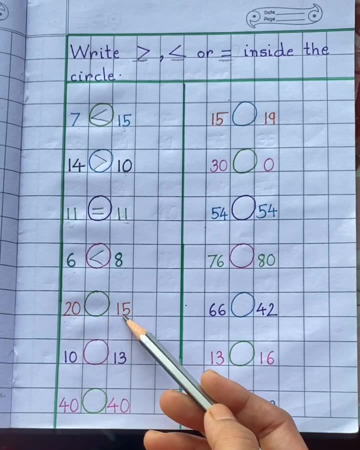 So we will put less than sign. 6 is less than 8.. Now look at these two numbers: 20, 15.. While comparing these two numbers, which number is greater? Yes, 20 is greater, So we will put greater than sign. 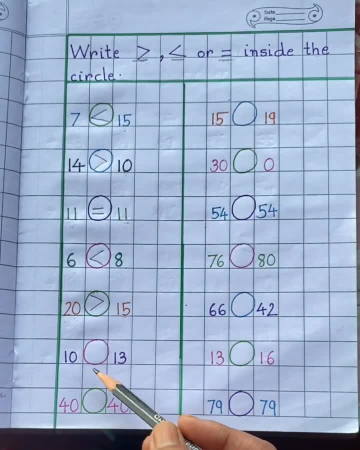 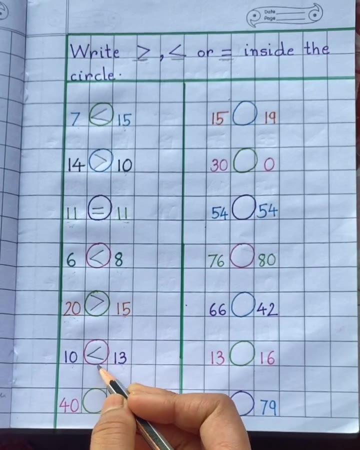 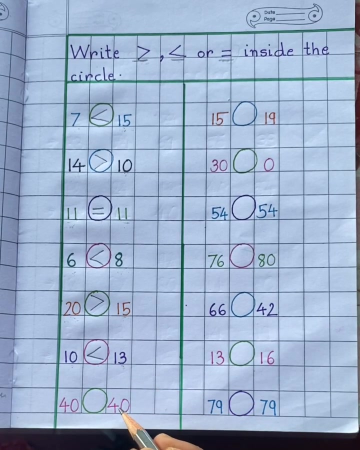 20 is greater than 15.. Next 10, 13. Which number is greater? 10 is greater than 13.. So we will put greater than sign. 10 is greater than 13.. 40, 40. Both the numbers are same, So we will put equal to sign.